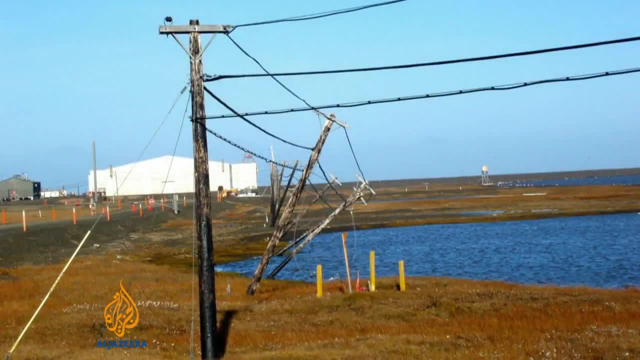 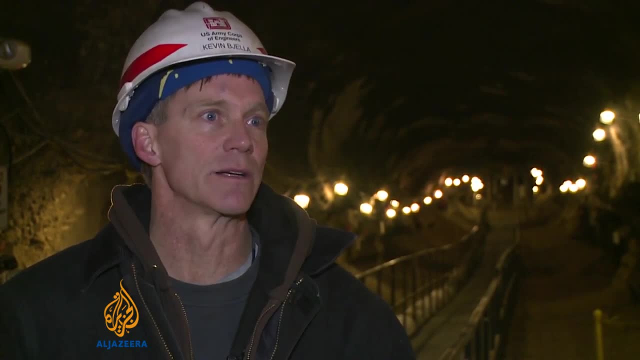 and how it's probably going to get worse. The idea is not to scare anybody. it's not to set a you know, set out this, this notion that everything's thawing and we need to stop burning gasoline. That's not what we're talking about. We're just talking about trying to 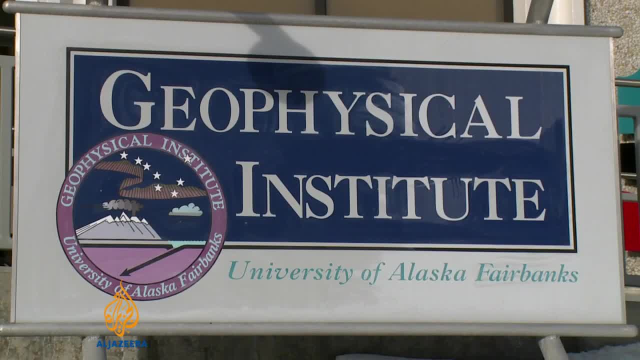 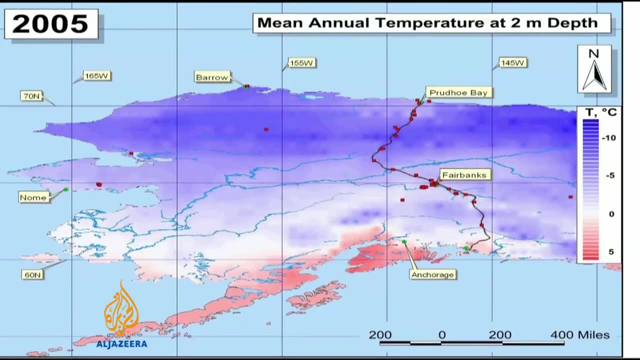 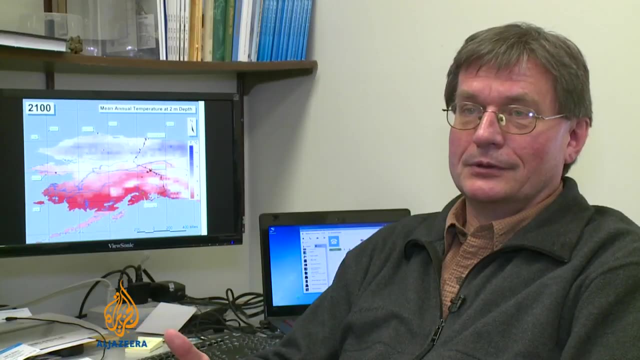 anticipate changes. There's real alarm among scientists. Permafrost is warming rapidly. Even worse, a huge amount of carbon is trapped in the frozen ground, Those plants and animal bones, and that will be released into the atmosphere as it thaws. Warmer climate will be more permafrost thawing, producing more. 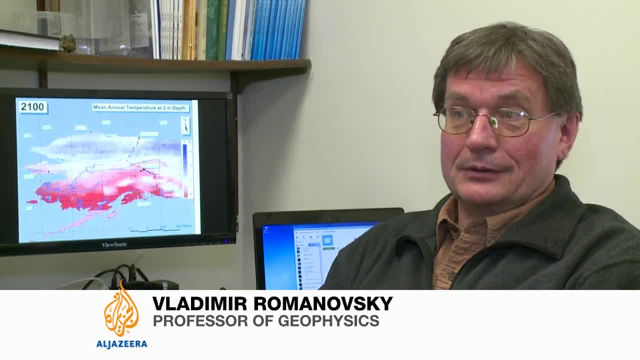 greenhouse gases, increasing this greenhouse effect, which will increase temperature again. And then we're going to have more permafrost thawing, And then we're going to have more permafrost thawing, And then we're going to have more permafrost thawing, And then we're. 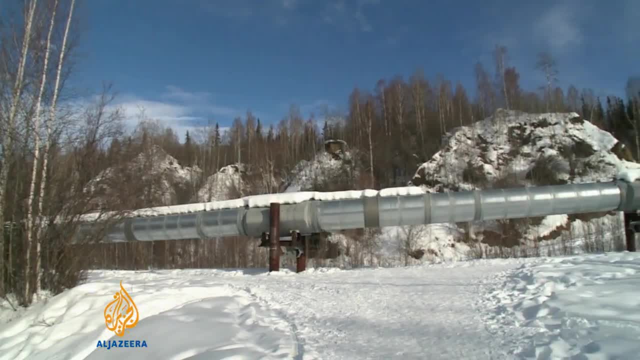 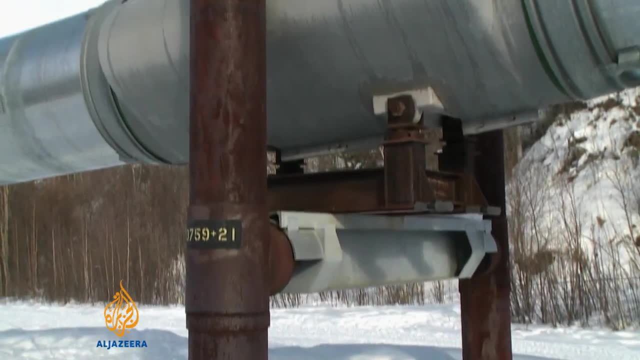 increased temperature, we'll thaw more permafrost. When the Trans-Alaska pipeline was opened in 1977, no one expected a changing climate, but they put the pipe on stilts to meet environmental regulations protecting the tundra and forest. So the way this pipeline is. 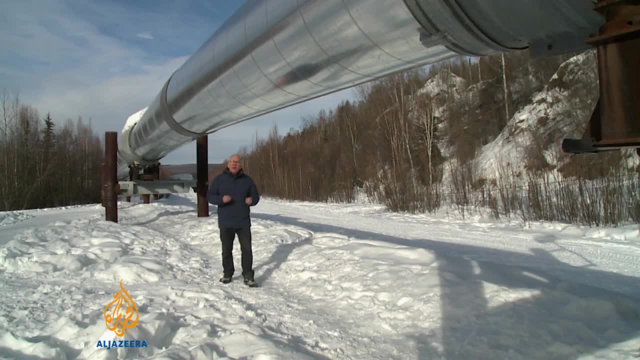 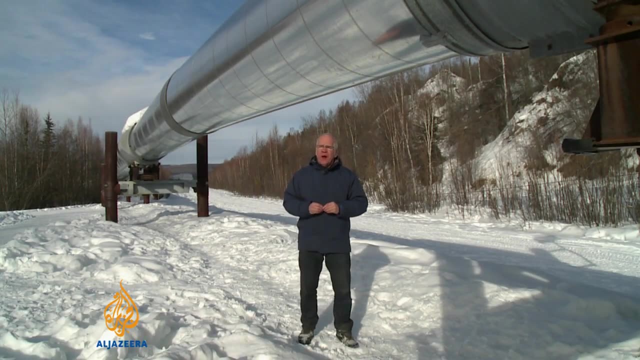 constructed that prevents permafrost from melting locally, but it's what's inside the pipe: Crude oil and its consumption, The impact of that on the world's permanently frozen ground- those are the much larger issues that government made up for. scientists and the planet have to consider. 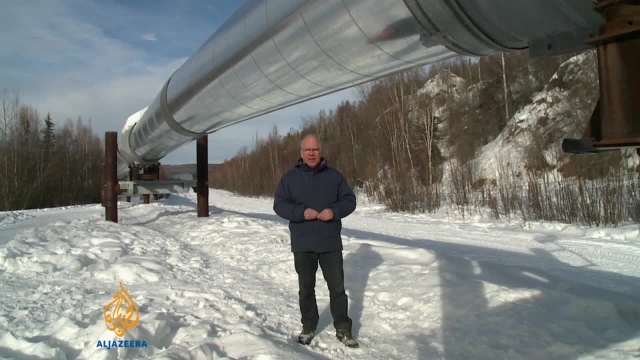 Daniel Lac Al Jazeera outside Fairbanks, Alaska.